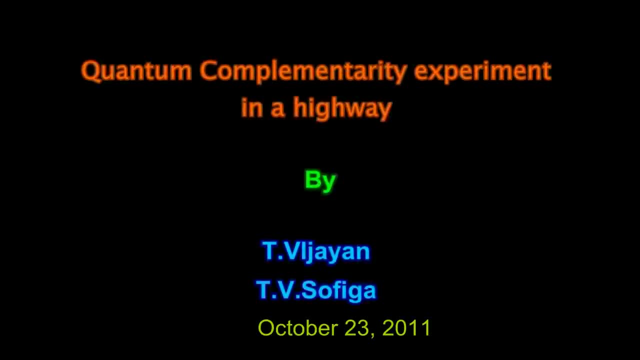 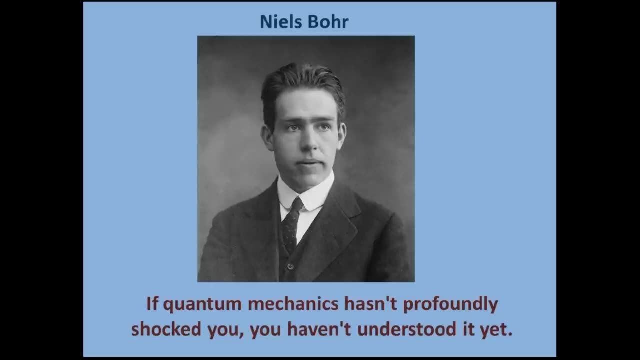 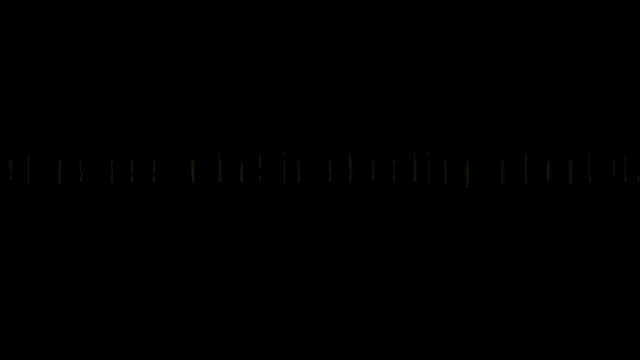 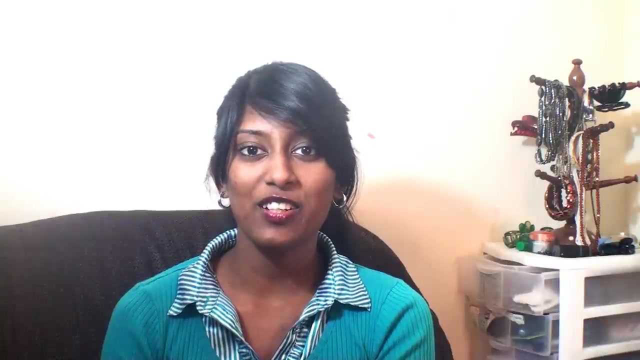 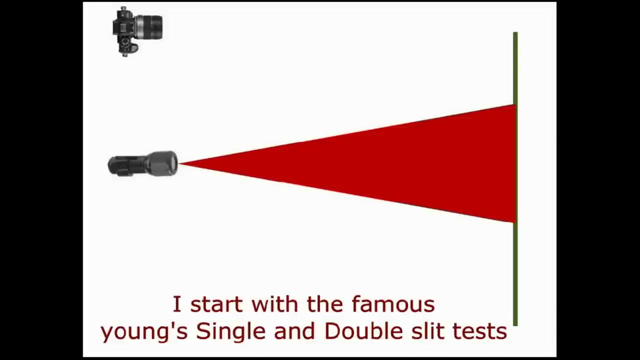 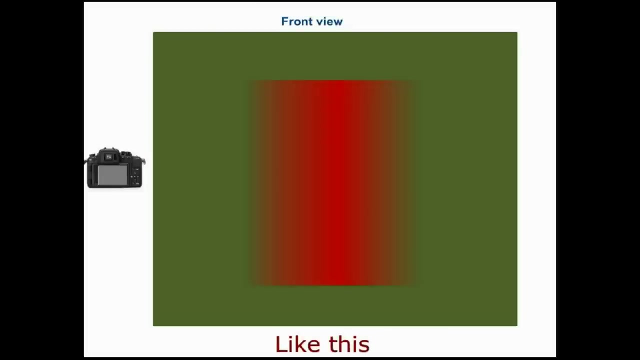 If quantum mechanics has not shocked you, you have not understand it yet. Let's start with Thomas Young's famous double slit experiment. His experiment proved that light is a wave, A wave is a Ergebnis, time is a set of functions And a wave is a set of functions. 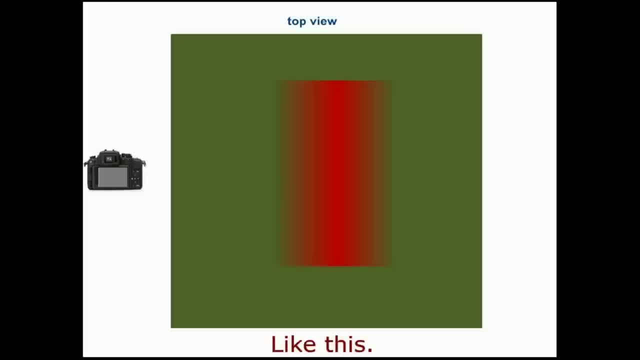 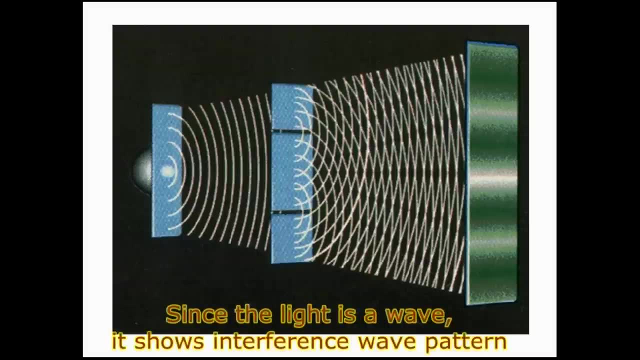 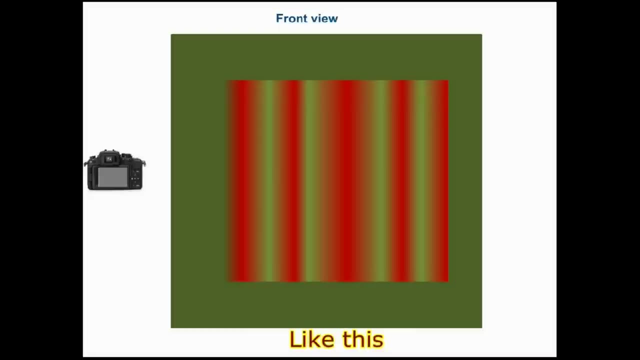 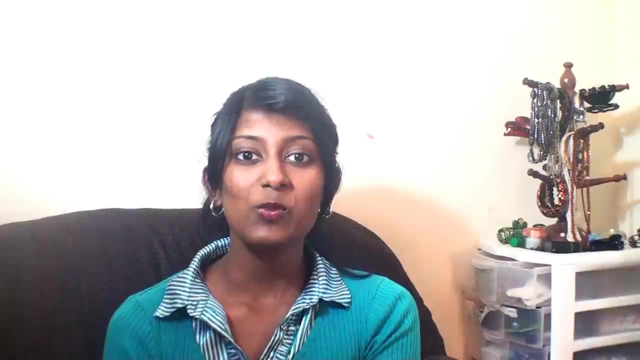 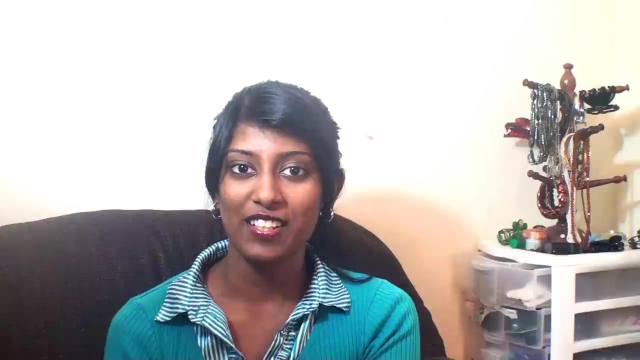 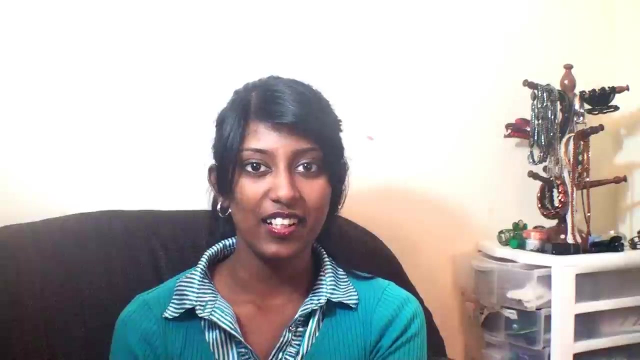 Now let's see where the wave is going. The wave is moving from a light source, Is it a point? No, Then the wave is moving from a light source to a. We just did the double slit experiment with light. Now let's see what happens if we do it with a single photon at a time. 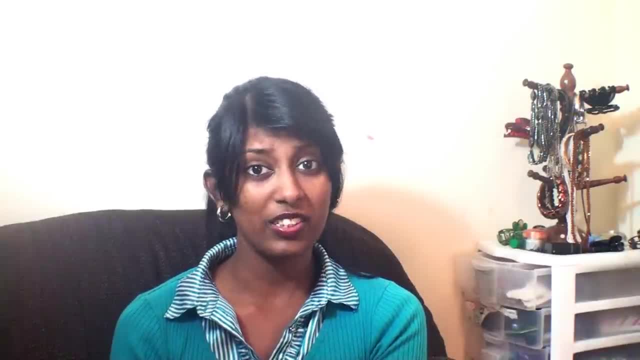 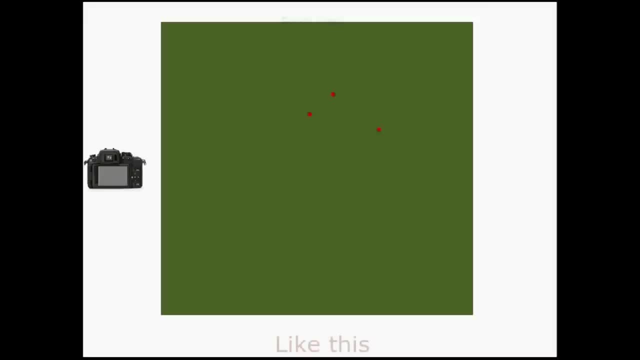 We cannot say for sure where the photon will go. It might go through the slit or it might not. Even if it does go through the slit, it's pretty hard to say where it will stop at. on the second screen, We cannot expect a wave pattern yet, because only one particle has been set. but after 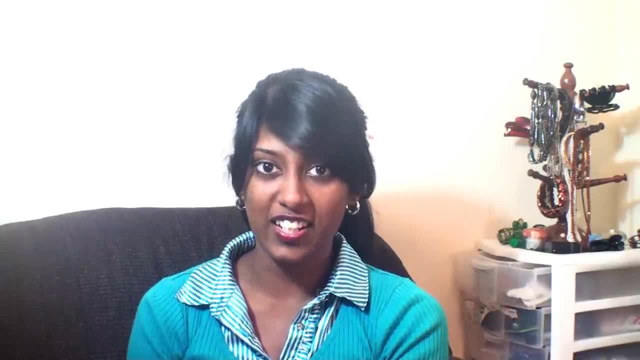 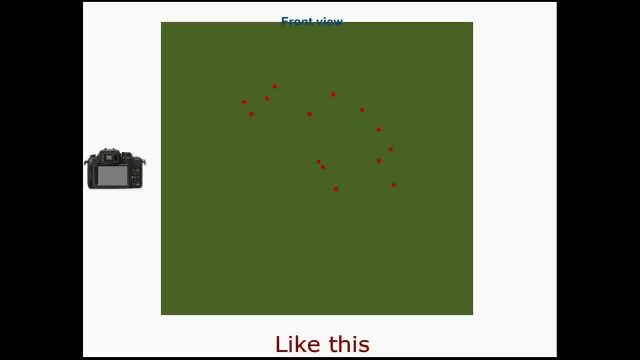 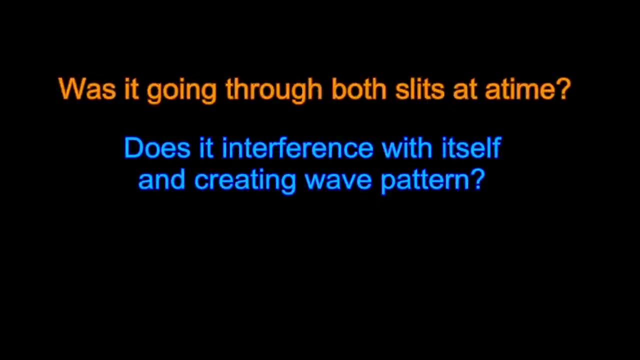 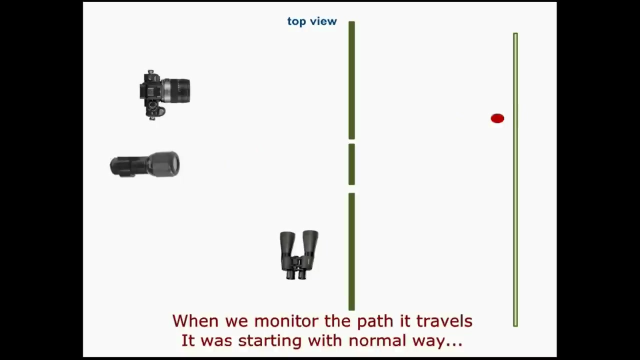 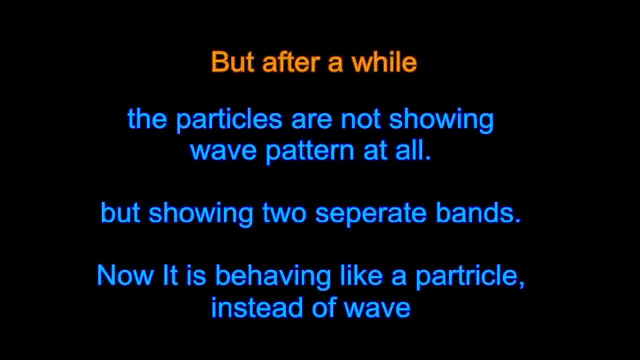 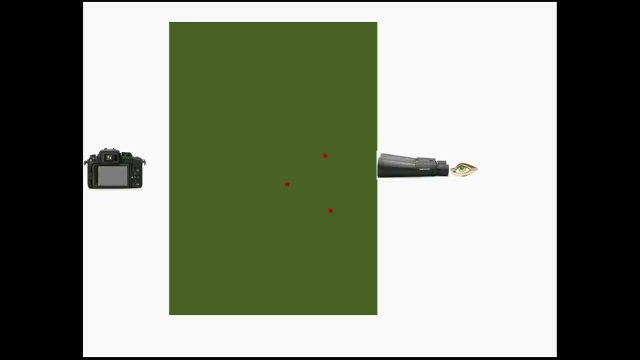 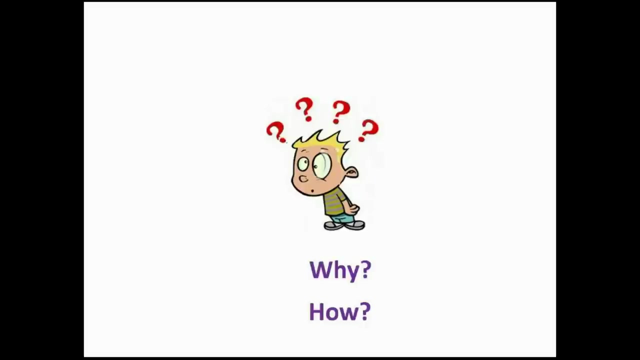 a while as more and more particles pass through the slits and onto the second screen. eventually, they will form a beautiful wave pattern. How'd it happen? Let us carefully observe the photon to see where it's going, Thank you. Now it's behaving like a particle and not a wave. 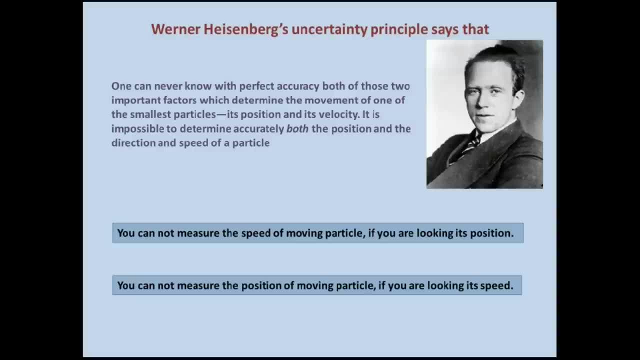 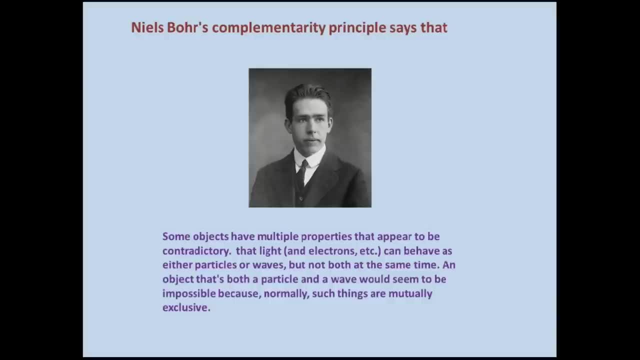 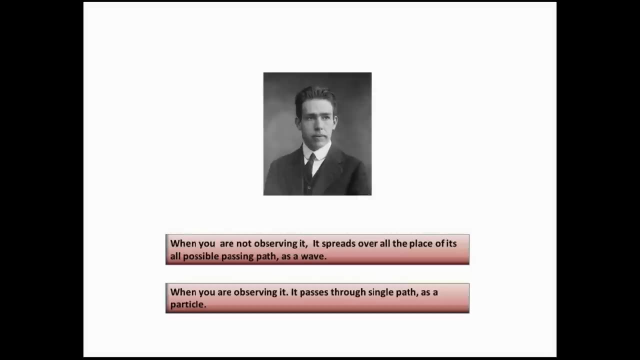 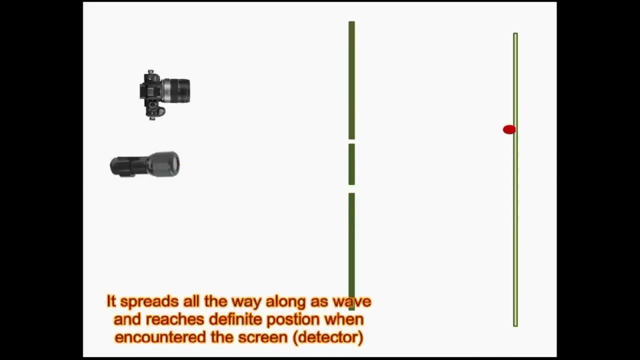 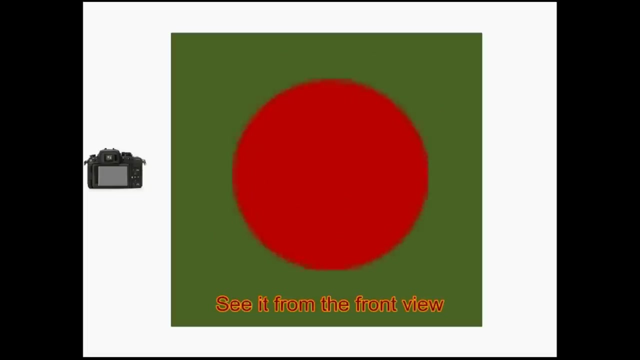 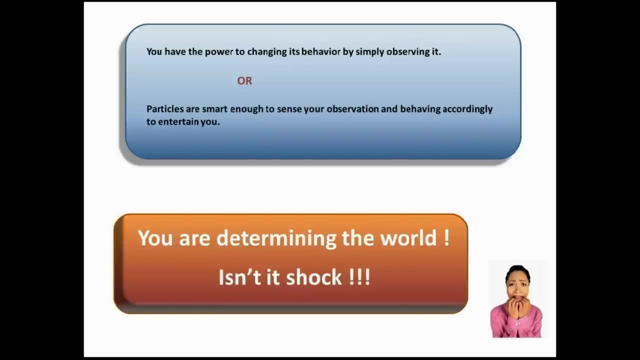 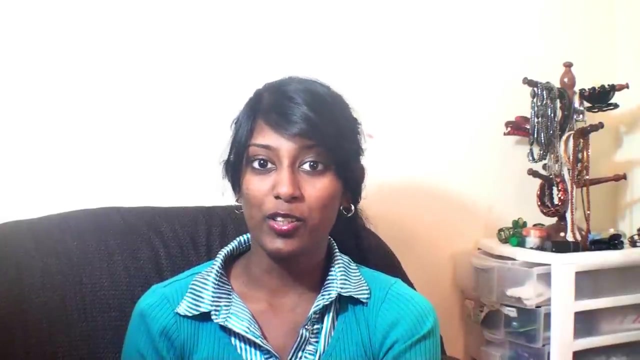 So wait, it's not a wave. then You have the power to change its behavior by just observing it. Either that or the particles are just smart enough to slender the particle and then change its behavior. So let's observe it. It makes sense that you are observing them and it's just playing with you. 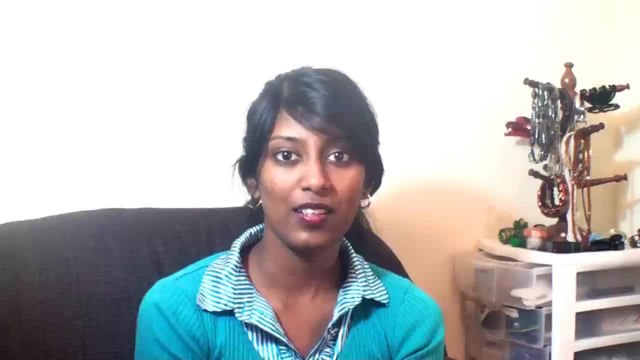 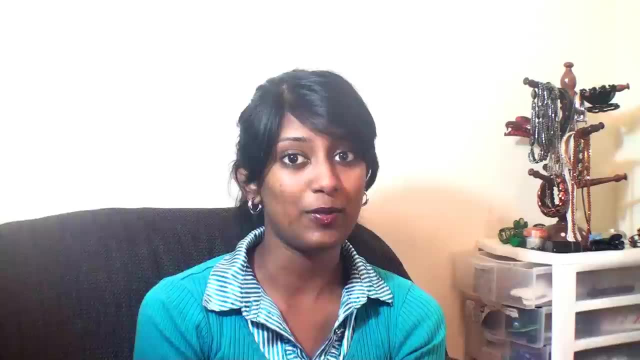 You're literally determining the world. Isn't that a shock to you? To clear ourselves on the complementarity principle, we can do an experiment of our own. For this experiment, you need a really fast-moving object to observe. Let's go to a highway where we can see fast-moving cars. 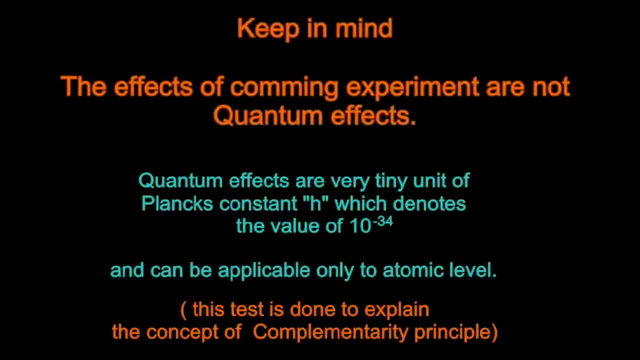 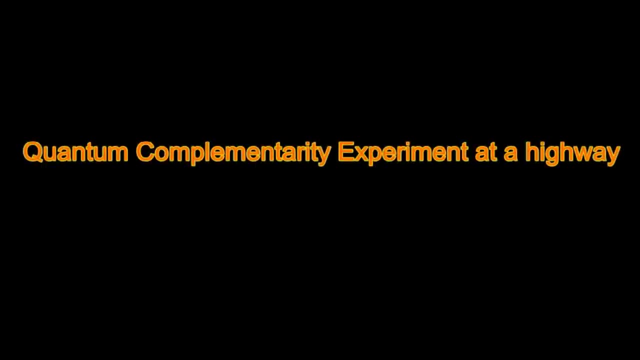 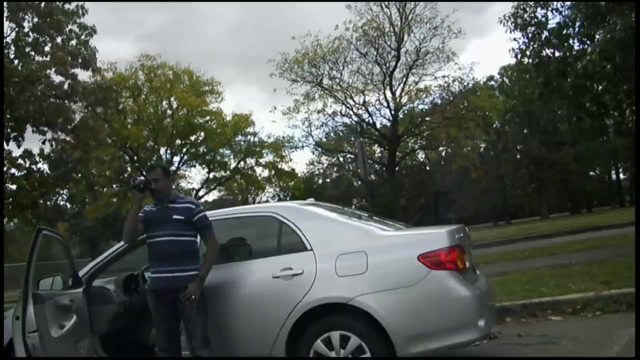 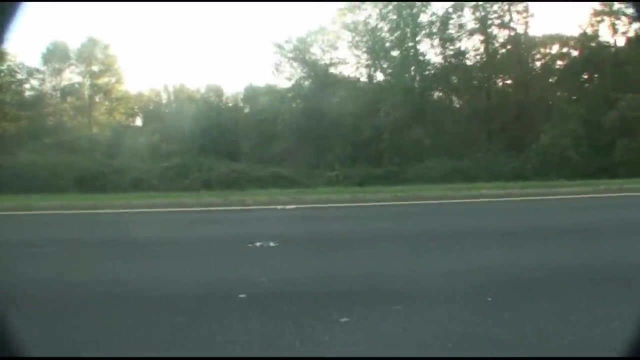 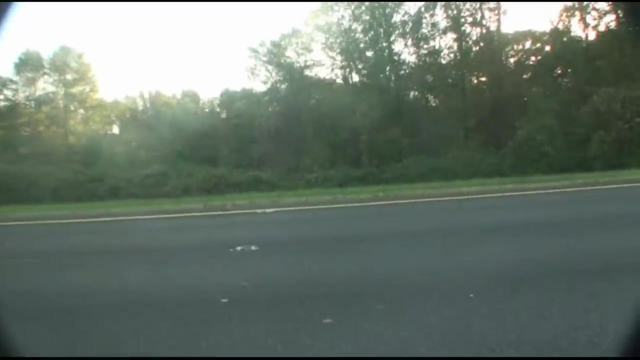 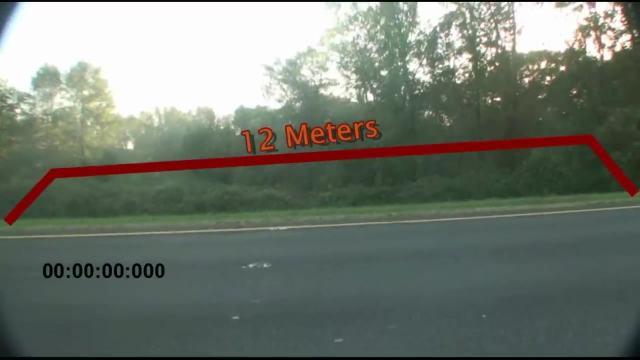 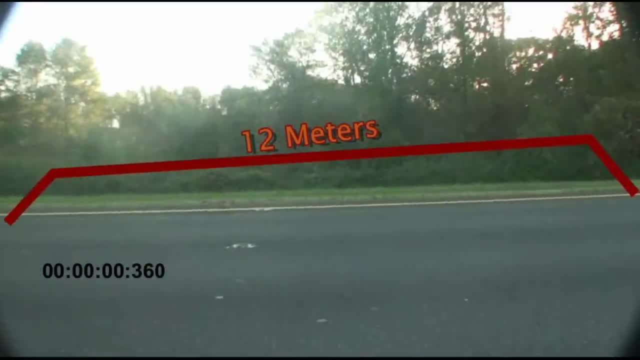 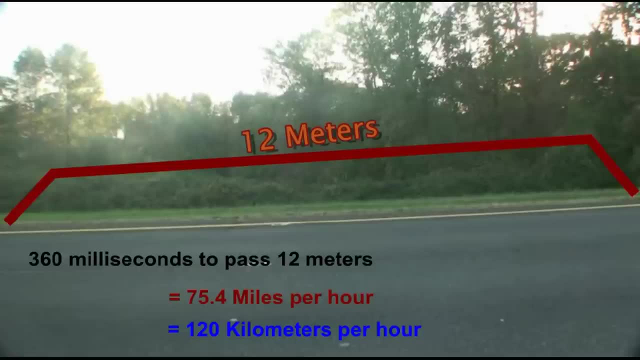 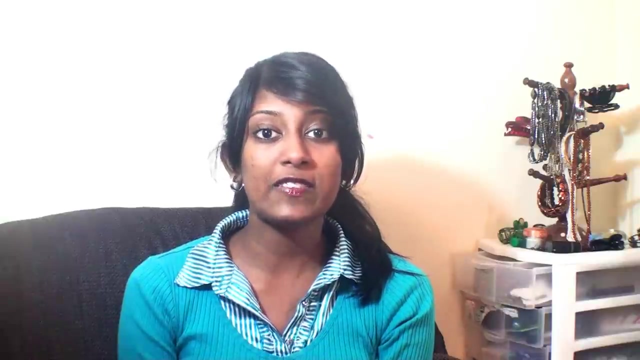 Let's go to a highway and just simply observe the cars. Let's go to a highway and just simply observe the cars. It takes the car 360 milliseconds to pass a distance of 12 meters at a speed of 75 miles per hour. 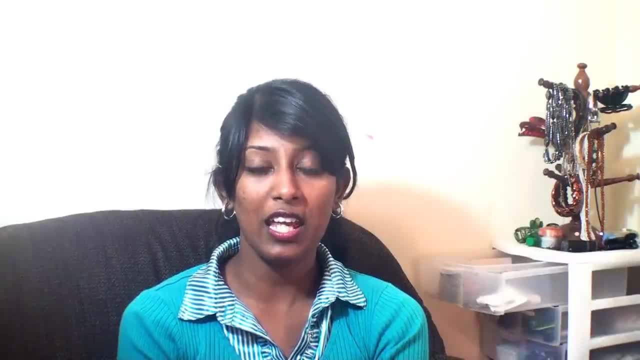 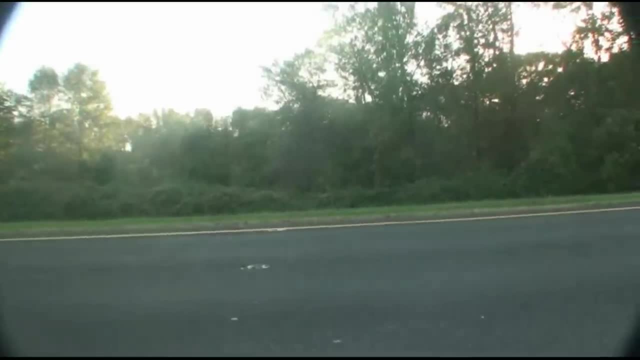 It is easy to find the speed of the car because both the beginning and the end points are stationary. Good, we found the speed, Now let's find its position. Oops, We missed it, So now let's try and freeze the frame. 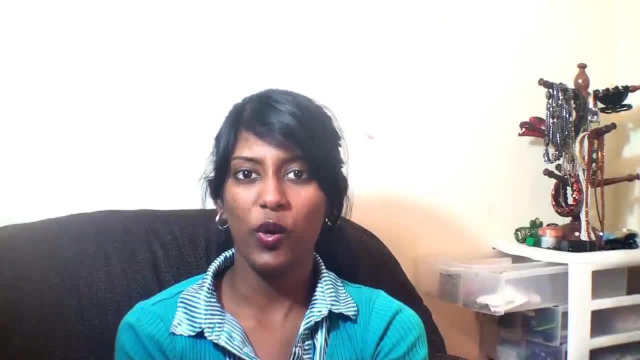 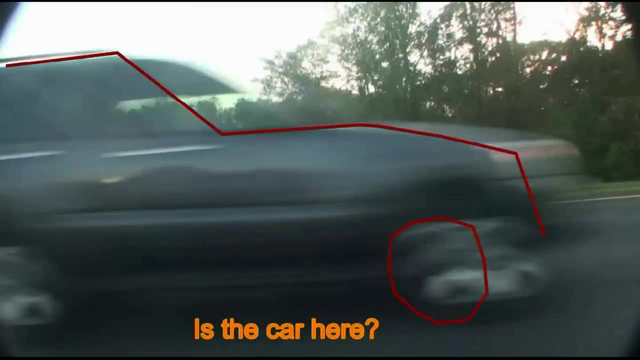 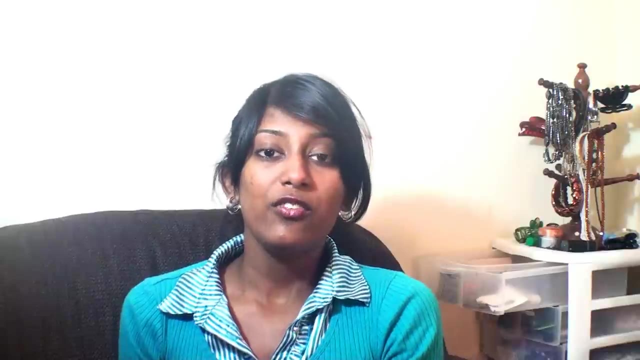 Yes, We got it, But hold on, Where is the car exactly? Is it here Or is it there? When you freeze the frame, it looks like the car was pulled. It looks like the car is in several places. This is called superposition. 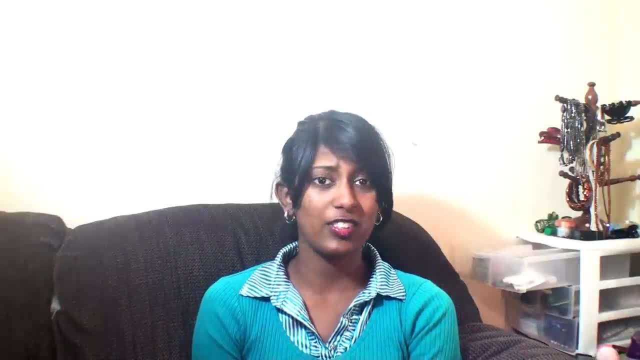 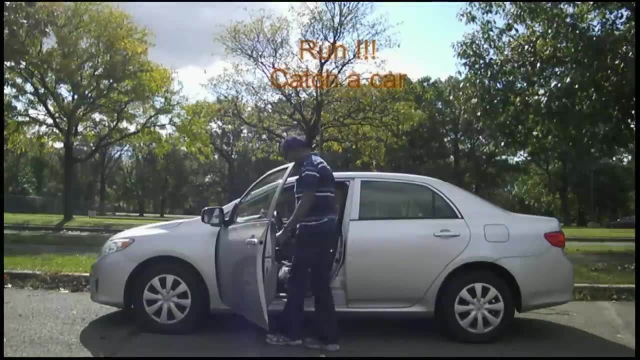 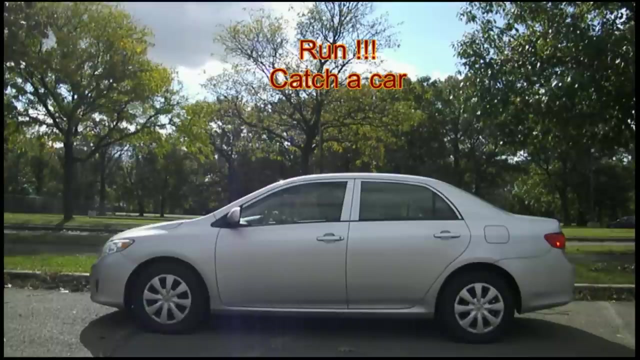 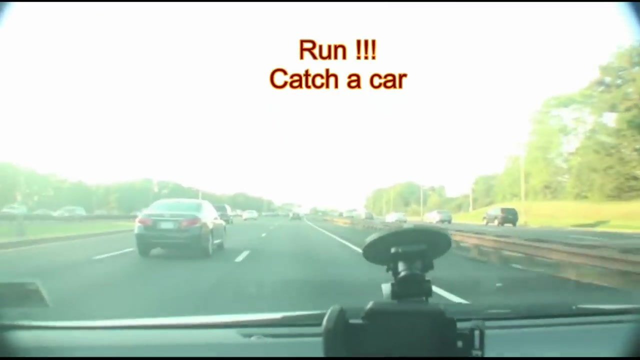 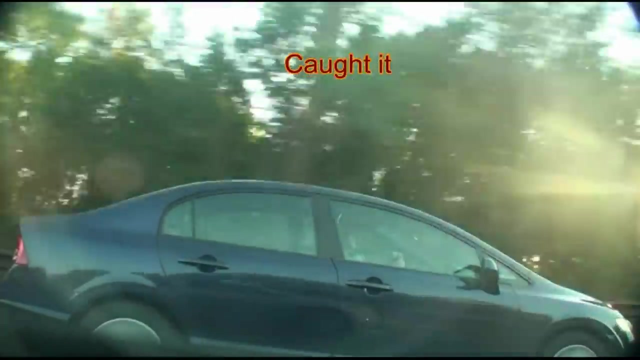 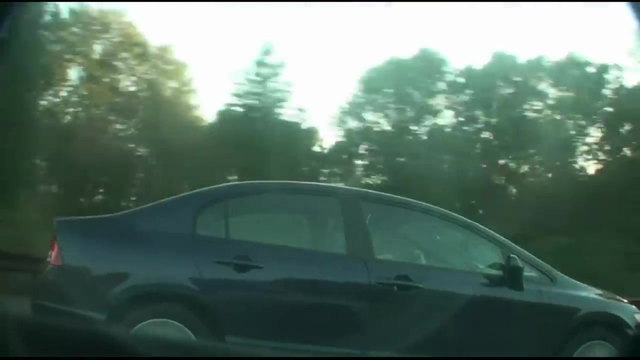 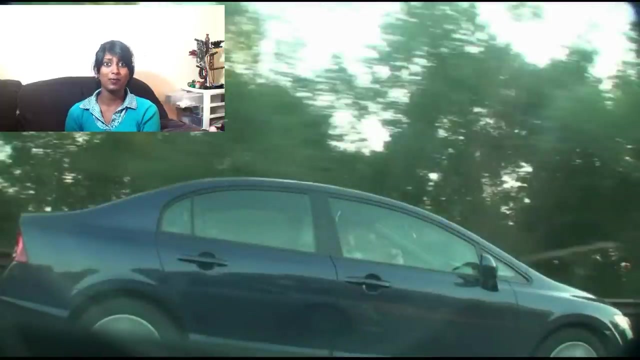 How are we supposed to figure out the position while the car is in many places? So why not just try and follow the car? Catch up with the running car. Now let's see the position. Freeze, please. Great, We found the exact position. Now what's the speed?